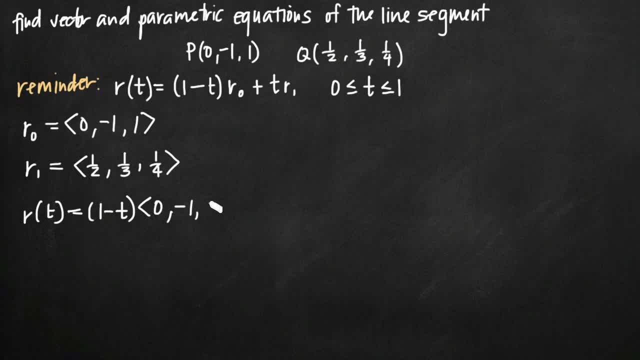 we plug in our vector r sub 0, so we'll say 0, negative 1, positive 1, plus we multiply r sub 1 by t. so we have this t out in front and we multiply it by the vector r sub 1,. 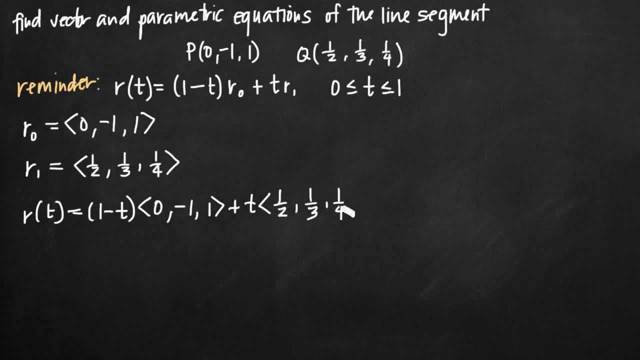 1 half, 1 third, 1, fourth, like this. Now we just need to simplify this, and simplifying is as easy as distributing this 1 minus t across each of our vectors: r sub 1 and r sub 1,: 1 half, 1 third, 1 fourth. So here's what that looks like, Multiplying 1 minus t by: 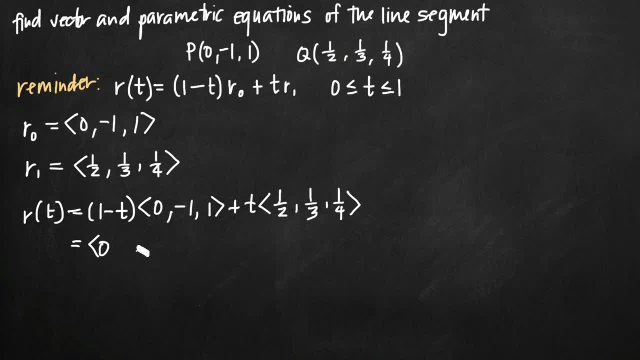 0 is obviously just going to give us 0. Multiplying 1 minus t by a negative 1 just gives us a negative 1 plus t. This negative 1 changes the signs on both of these values here. so positive 1 becomes a negative 1, negative t becomes a positive t, And then 1 minus t. 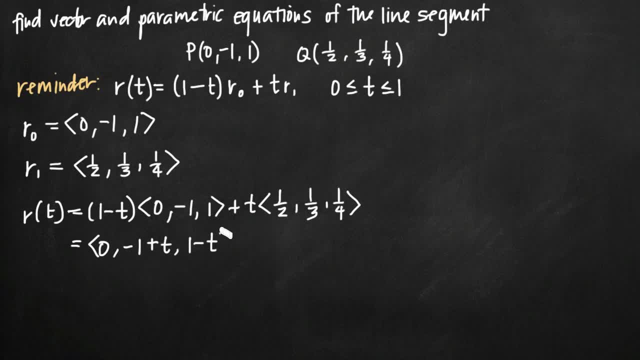 multiplied by 1 minus t is equal to negative 1 plus t. So we're going to multiply this 1 minus t by 1 is of course just 1 minus t. So we distributed that. now we just need to distribute our t across this second vector. So we're going to get the vector here 1 half. 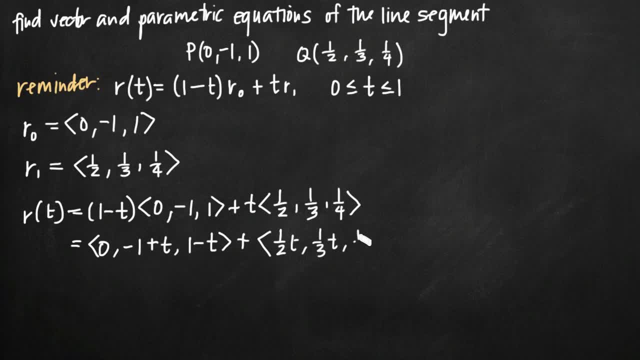 t, 1 third t and then 1 fourth t. And now, because we've essentially added two vectors together, we just have one vector added to another. we're just dealing with vector addition and we can add each of our components together. So, adding our x components together, 0 plus. 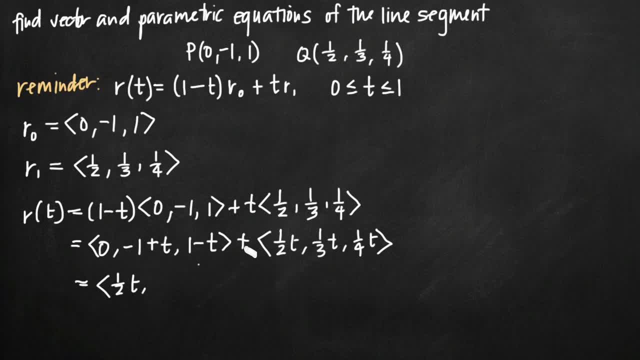 t. 1 half t just gives us 1 half t for our x component. For our y component, we want to add negative 1 plus t to 1 third t. We've got our negative 1 out in front. then we just: 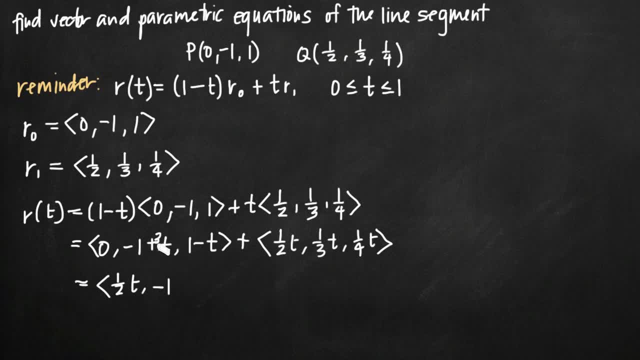 get t plus 1 third t. Think about this t here as 3 over 3t. so when we add it to 1 third t in our numerator, we're going to get 3 plus 1, or 4, and we have our common denominator. of 3.. So we're going to get 4 thirds t, so negative 1 plus 4 fourths t. So we're going to add our negative 1 plus 1 third t to our third t And we're just going to add negative. 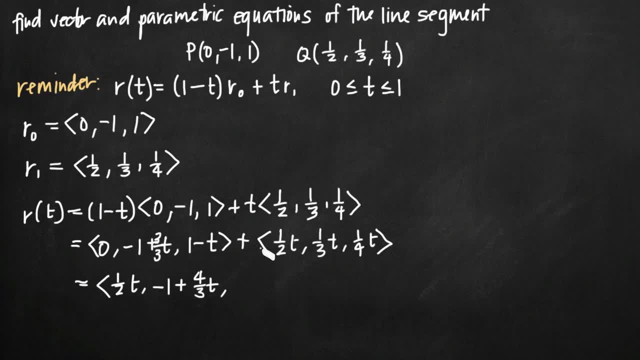 4 3rds t, like this, And then for our z component, 1 minus t plus 1 4th t. we've got our 1 hanging out in front here, and then we have here a minus 4 over 4 t, negative 4 over 4 plus a.